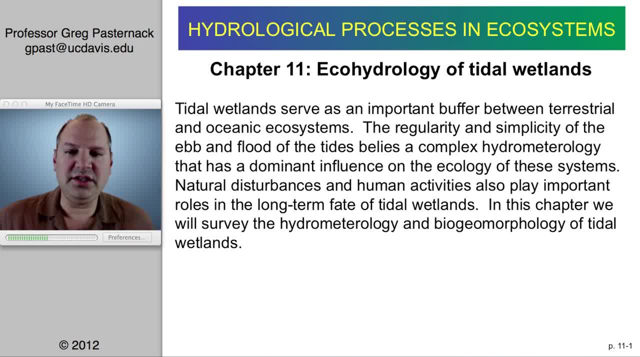 This is the first video podcast for Chapter 11 on ecohydrology of tidal wetlands. Now, all of the different classes within the hydrogeomorphic classification have a lot of merit and they all deserve study, But of them all, tidal wetlands have probably received the most study, and for good reason, since the majority of humans live near coasts. 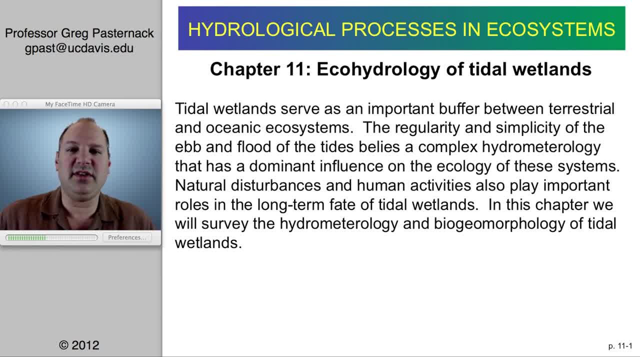 Wetland conditions have long affected human civilization. In the modern era, scientists have likewise lived in coasts and spent a lot of time trying to understand them, and so tidal wetlands have been very important. You know, a lot of rivers drain to the ocean. well, they all drain to the ocean, of course, but a lot of them are buffered by having large wetlands between the river and the sea. 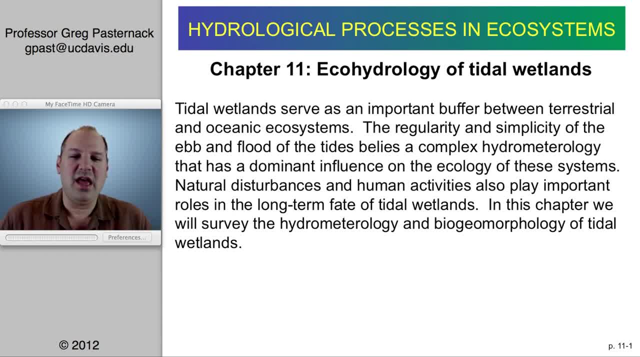 usually fringing an estuary of some kind, but not always. And you know, one of the things that's hydrologically interesting is that, because tidal wetlands are so important, because tides represent a regular periodicity, as you'll see, of having flow coming in and out, 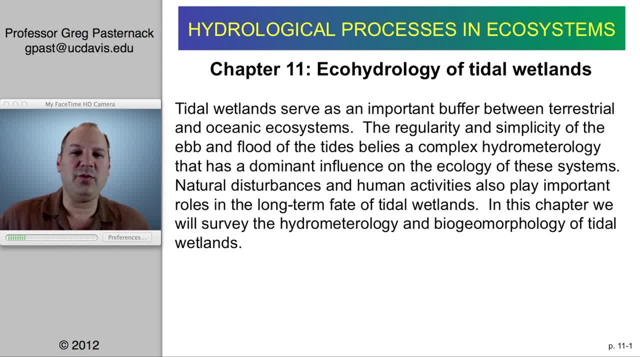 you know, in contrast to rain-driven events, it really creates what ought to be a relatively straightforward analysis of what's going on. However, as you'll see, there's a lot of complexities in terms of geomorphic impacts of human activities and disturbances. 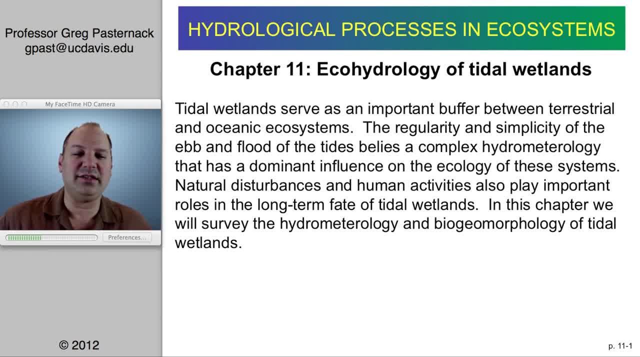 and hydrologic impacts of things like winds or hurricanes, So there's a lot of complexity that's at work In coastal wetlands and as a result of that, it's worthwhile to take the time to try to understand the hydrology in more detail. 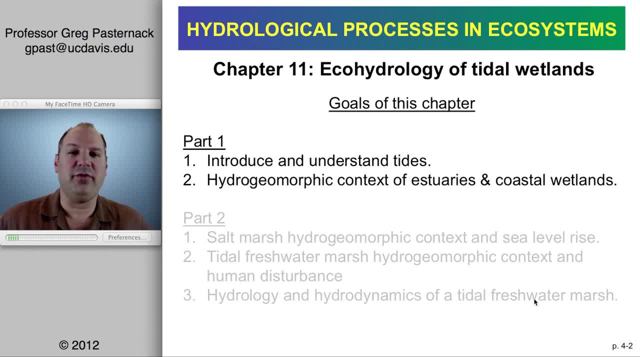 The goals of this first video podcast are going to be twofold: First, introduce and understand tides and second, let's look at the hydrogeomorphic context of coastal wetlands, but focusing on the larger estuarine and coastal context. 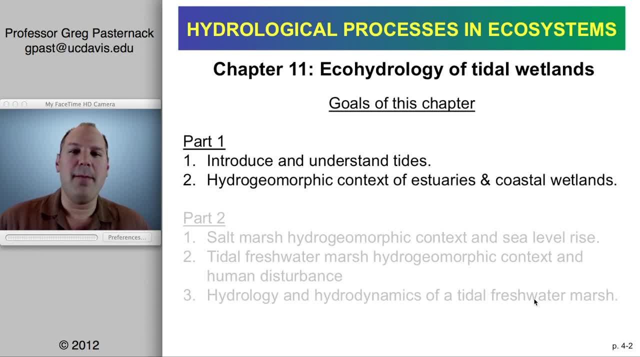 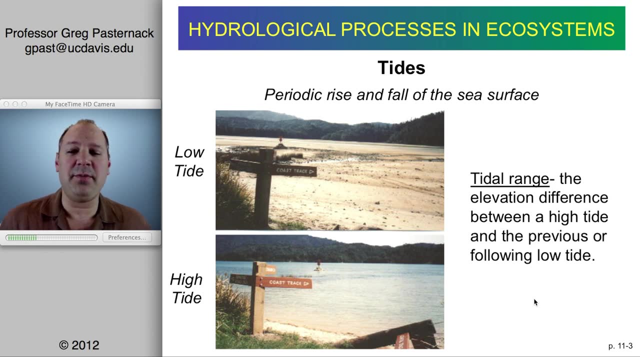 I'm not going to go a lot into the geomorphology of coasts, but we will look at the broad context, because these wetlands tend to occur across the gradient, within estuaries and near them. Okay, tides- The definition of a tides is very simple. 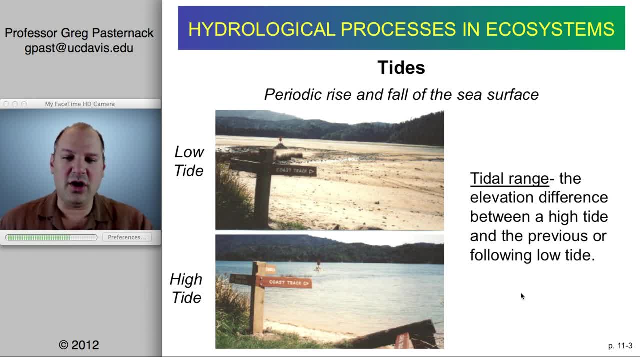 Periodic rise and fall of the sea surface. In the top photo you see exposed soil and in the bottom photo you see water. The photo is taken at the same location. The water has come and gone through these photos and that's the top. 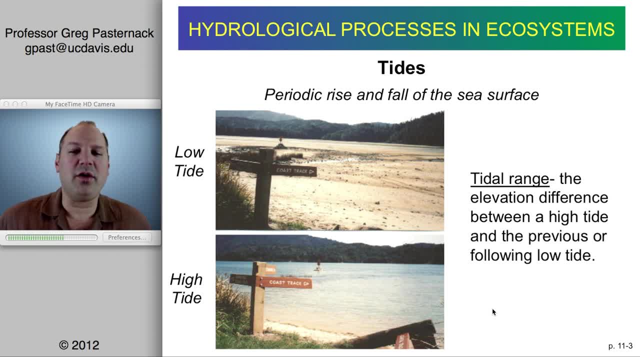 The first thing we want to look at is the tides. We can define a quantitative property known as the tidal range or amplitude, which is the elevation difference between high tide and then the next or immediately preceding low tide. So we can see that elevation difference and take note of that. 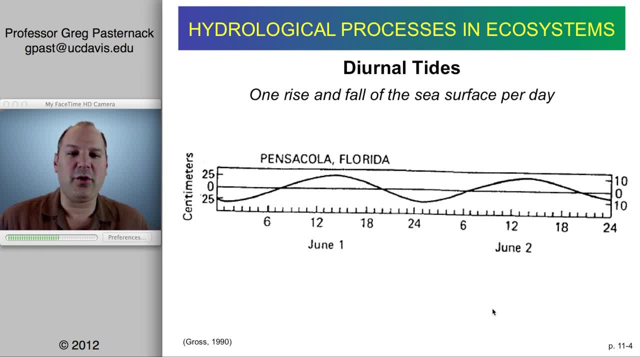 Tides come in a whole bunch of different varieties. The first is when you have one rise and one fall of the sea surface over a 24-hour period. So if we look at this day, here's 24 hours on the x-axis. the y-axis is elevation from 25 centimeters below mean sea level to 25 centimeters above mean sea level. 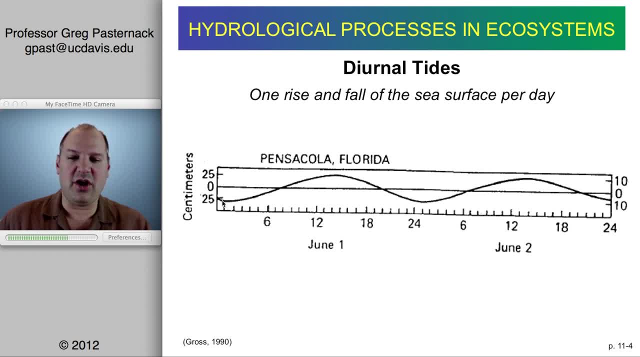 And what you can see is that the tides start off- in this case low cross mean sea level here- rise back up and then come back down 24 hours later. So over a 24-hour period, you have one low tide, one high tide and you're back to where you started. 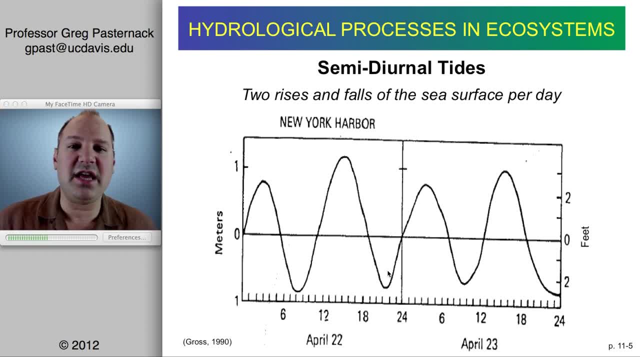 A semi-diurnal tide is the same idea, but you just get two of them in a 24-hour period. So, starting in this case from mean sea level, we rise to a peak, drop to a low rise, again, drop again and get back to where we started. 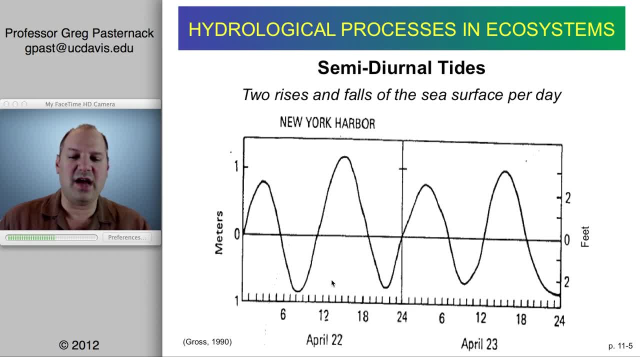 In this case, you can see that the high tides and low tides are relatively similar to each other. So we just call The top of this curve the high tide and the bottom the low tide, And then this line in the middle represents the long-term average sea state, or what we define as mean sea level. 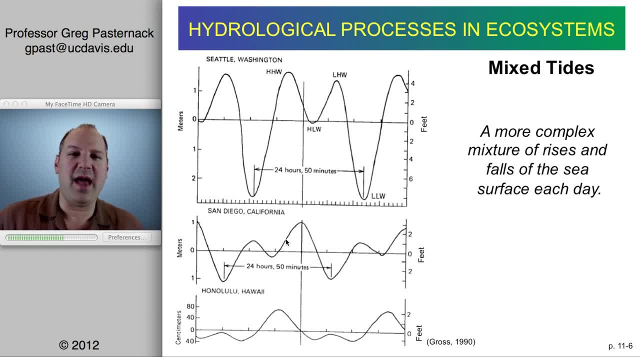 There are also places that have mixed tides, and San Francisco Bay is one of those regions. So if you look at tide tables for this area, you'll see this effect. So we can start here again over a 24-hour period or so. 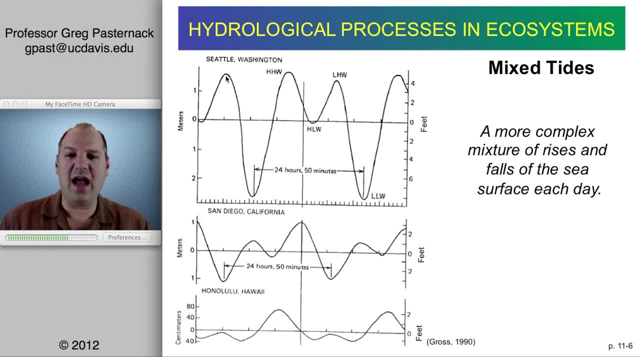 You have started around mean sea level. Then we hit a high tide, Then we hit a very low, low tide, Literally a low, low tide. Then we go up and we hit an even higher high tide. So you say a high, high tide. 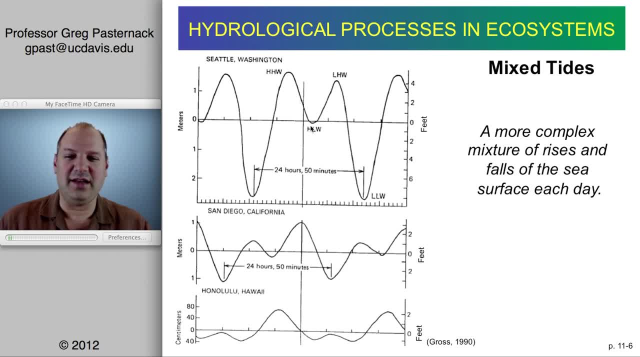 And then we have a high, low tide, Then we have a low, high tide And then we back to the low, low tide again. So I went beyond that. But the point is that it's mixed in, that you have this very confusing. you know the two highs? 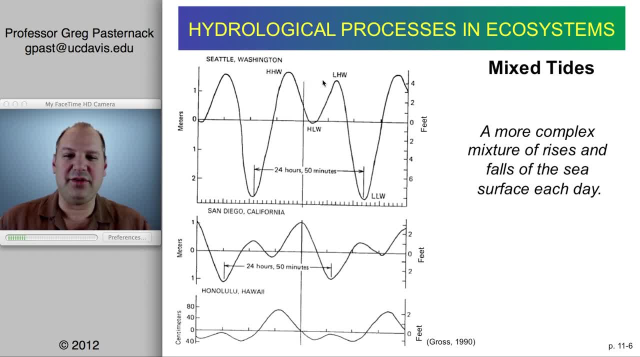 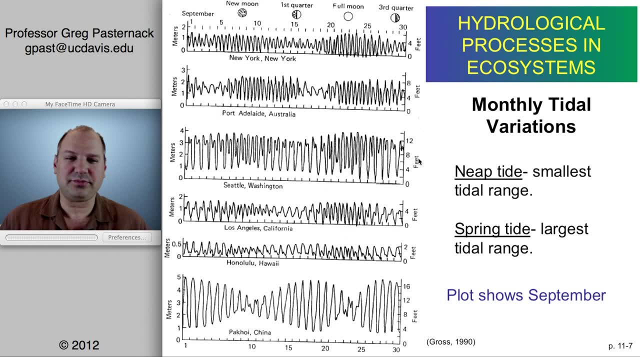 that you have a day are high, but they're not as high. one is not as different than the other, and especially here on the low tide, so that's called the mixed tide. as if that's not complicated enough, we also have month-long tidal variations. what we 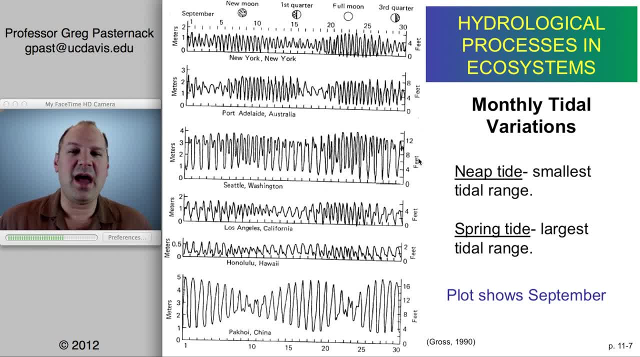 call neap tides and spring tides. neap tides are the time of the month when you have the smallest tidal range or amplitude, and spring tides are when you have the largest. so here I'll say a sentence that is very confusing. but what? 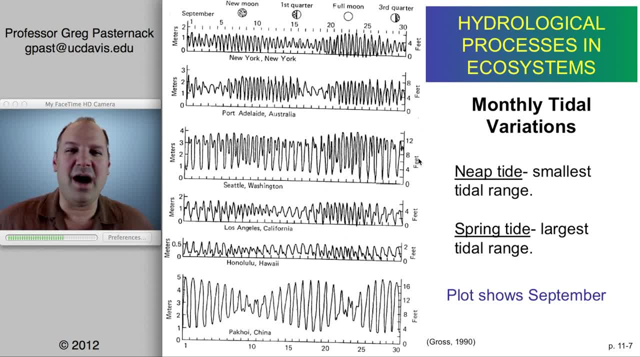 you're seeing here is a tidal modulation of the amplitude of the water surface. modulation is the key word. modulation means that we're not affecting, in this case, the frequency signal, we're just affecting the amplitude. so this variation in the vertical distance- here the tidal range, is the amplitude of the tidal range and the amplitude of the tidal. 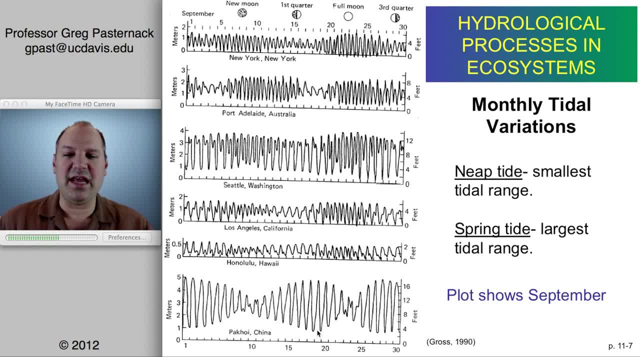 range. we could say that that's being modulated. this is the same as you could talk about any kind of periodic signal. so if we look at the bottom here, this is a tidal record from Pakhui, China, and you can see this large tidal range of going. 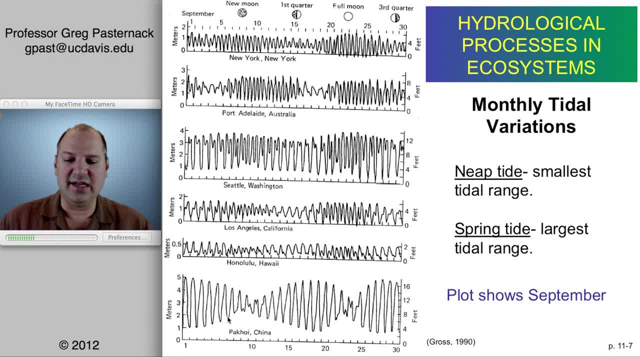 from 1 meter to 5 meters, so 4 meter tidal range. as the month goes on, we're 10 days in. this is days now on the x-axis and you have a very small tidal range. so we fit the neap tide and then it widens out again: spring tide, neap tide, spring. 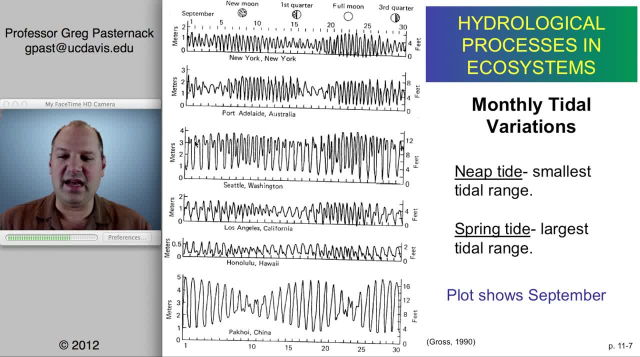 tide. if you look at these other signals where you have mixed tides, like Seattle Washington, it gets relatively complicated. but if you just zoom in, you know, you see, you see the detail, large tidal range. you know small difference between high, high high tide and high- low high tide, but there's still a big. 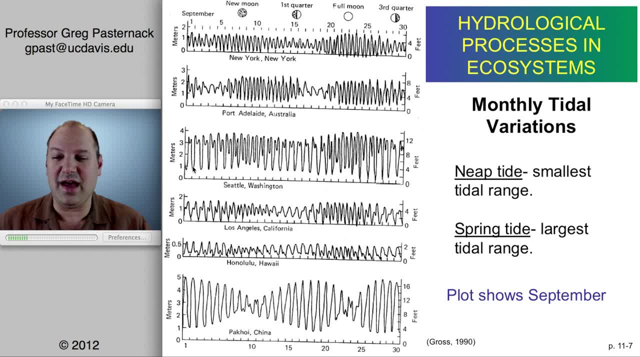 difference here between the high low tide and the low height, low, low tide. but by the time you get to the neap time you see that the overall tidal range is a lot lower. let's see, this is a little confusing. so then you come here and it. 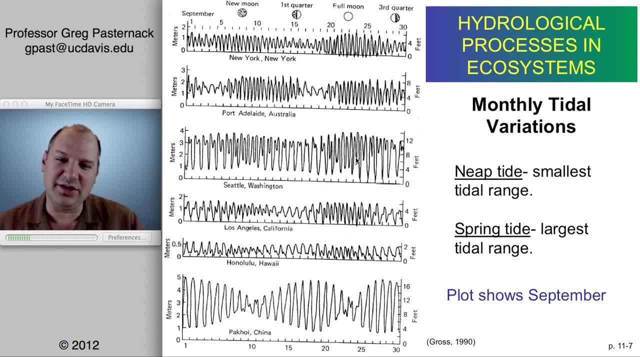 remains quite low, but then here widens out a bit, so it's a little bit. this one's a little bit confusing to see when, but this looks like the biggest tidal range here, which would make this a lower tidal range. so then it's kind of mixed and 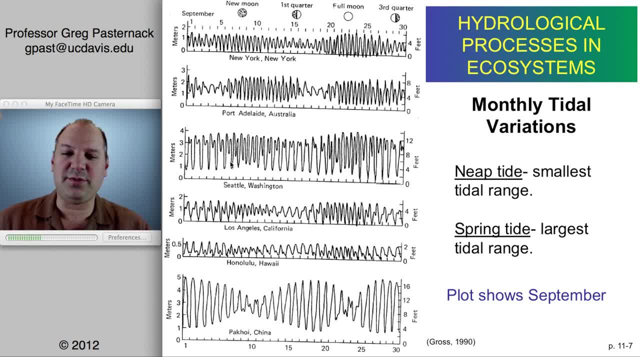 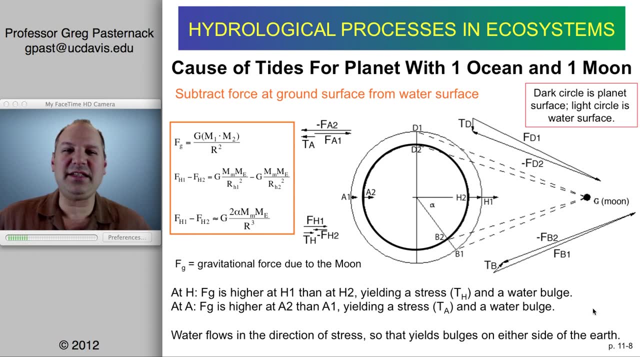 then it's supposed to be big again, so not the clearest of signals. but you can see, with a mixed tide it gets quite complicated. with these relatively simple semi-diurnal or diurnal tides it's much easier to see these modulations. so why do we have tides now? this is the most miserable. 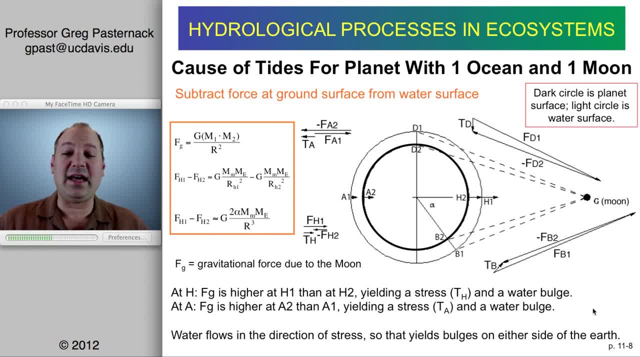 part of the whole thing and out of this whole class. this is the slide and the question that I find the most frustrating, and the reason for that is if you pause here and go on the Internet and say, why do we have tides, what you'll find out is that the Internet doesn't know why we have tides. there's all kinds. 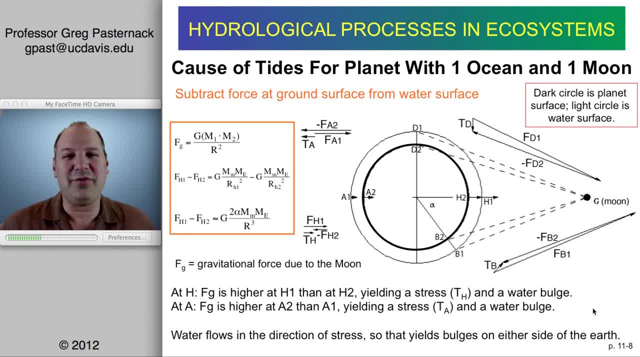 of things that people talk about. centrifugal force is centripetal forces, shear stresses, all kinds of things are talked about, and you'll see that, in fact, the explanation in a basic oceanography textbook is probably wrong, and a lot of the explanations on the Internet are wrong. 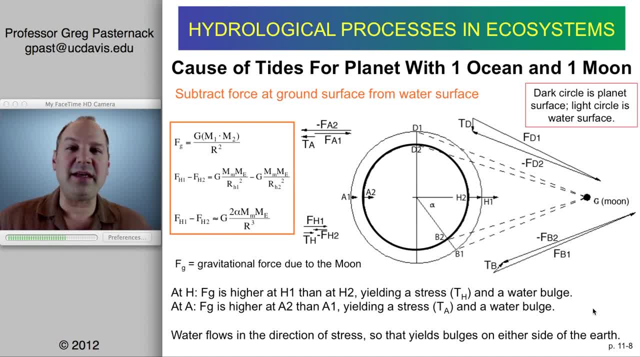 there's a lot of miscommunication. the best explanation I can find that satisfies my level of curiosity- which I pretty sure is correct but is also not so easy to grasp, necessarily- is what I've illustrated here, and I've tried to make it as simple as possible. and you can see it's not that. 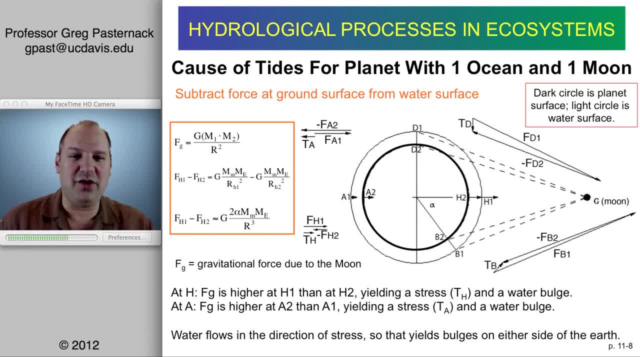 simple, but essentially, what we have is shown here is a solid earth, shown by this thick red circle. so imagine an earth and it's completely inundated with water, which is the thin circle around that. okay, so this is a water world, a pure round water world. this world has one moon circling around it and there is 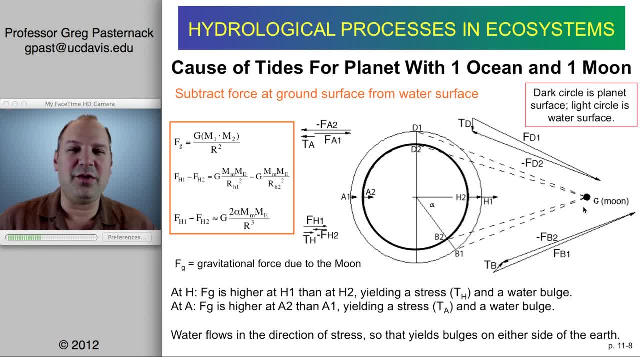 no Sun. so miraculously, there is liquid water on a round planet with no Sun and it has one moon. now what's happening is that we have forces that are being applied between any two locations. we can look at the force between the moon and any point located. 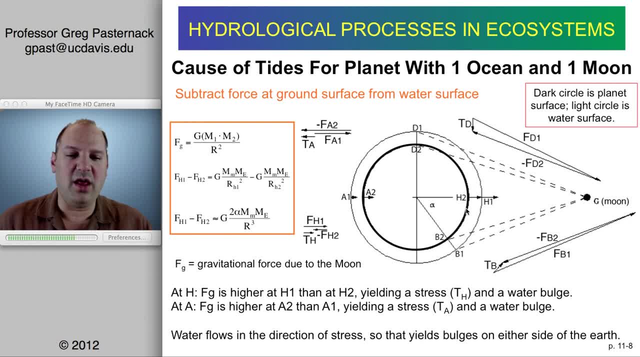 on the surface of the water as well as at the interface between the water and the solid ground. we have this gravitational force force equation that tells us that the force between these two objects depends on the mass of the two objects divided by the distance squared. In this case, the masses are pretty. 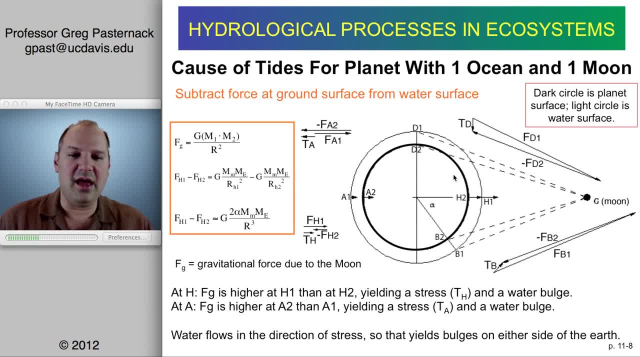 fixed, they're not changing. But if you look at the locations around the Earth, the distances between that location and the Moon are substantially different. And here's how it plays out: H1 is the point on the water surface closest to the Moon, Because it's the closest to the 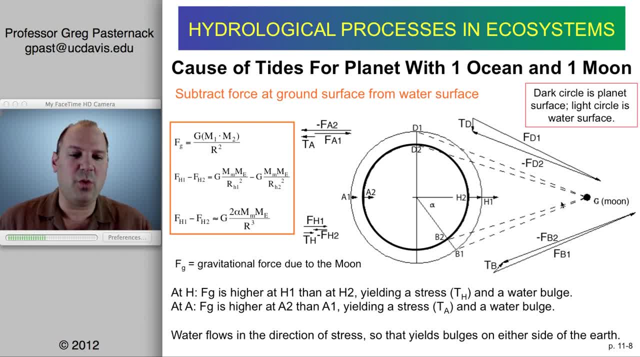 Moon. it has the strongest force between H1 and Moon, So therefore you can expect a very strong pull. Now let's look at H2.. H2 is far enough away that it's going to have a decreased force, And so the differential in force between H1 and H2, that difference between 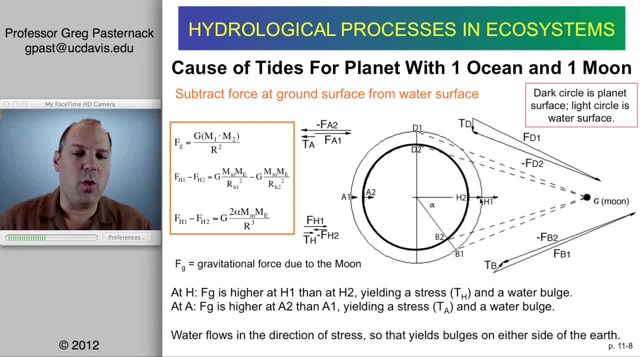 H1 and H2 is going to cause an apparent stress, in which water, you know, there's basically an apparent stress. so as a result of that, that means that water is going to have a tendency to flow from areas of less stress to areas of high stress. So if we look at D1 and D2,, 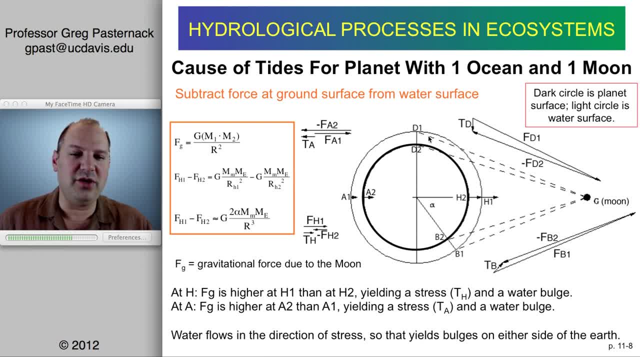 for example. whatever the difference is there between those two, it's going to be a lot smaller. You can see that the lines D1 and D2, they're relatively parallel. D2 may be a little bit shorter, But the differential between D1 and 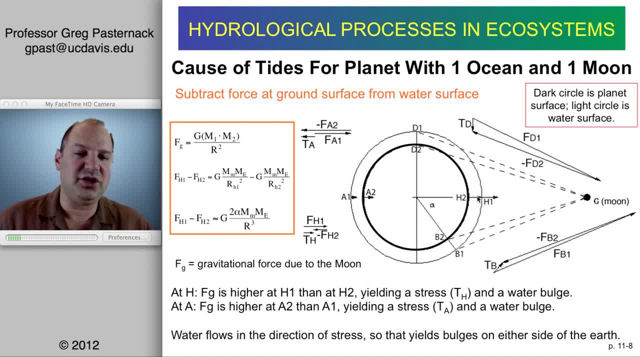 D2 is a lot smaller than the differential between H1 and H2. And that difference is going to allow the water to flow in the direction of the stress. Now let's come to A1 and A2.. Aha, I know what you're thinking. Well, A1 is really far away, so it probably has the 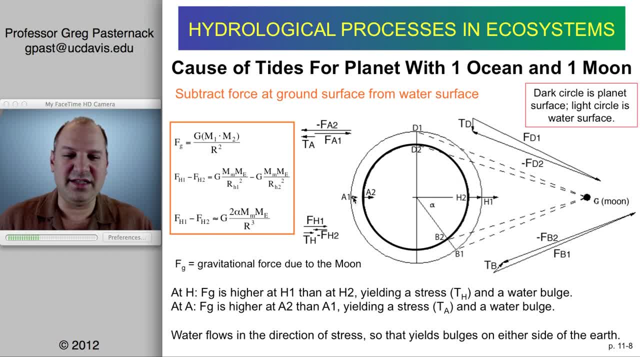 lowest of all forces. Yes, that's true. A2 has a little bit less force, So it's going to have a little bit more force. Now. A2 is a point on the ground surface, so the ground itself is not moving in this case, in any case, But there's a very large differential. 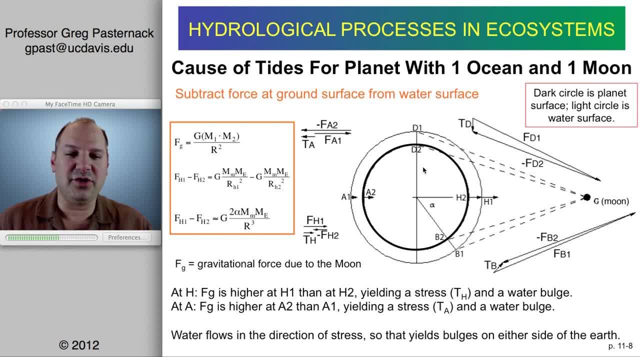 between A1 and A2, and it's a bigger differential than the difference between D1 and D2.. And so, in the same way that water would flow from the area of low differential to high differential, it will now flow from low differential to high differential this way. 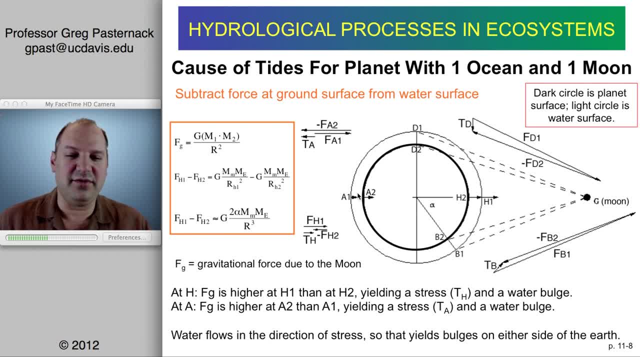 Now forget all these things about centripetal forces and all kinds of zany ideas. The bottom line is that, just as a function of distance from the moon, there's differential gradients, and that means there's differential stresses And water is going to flow from the area of. 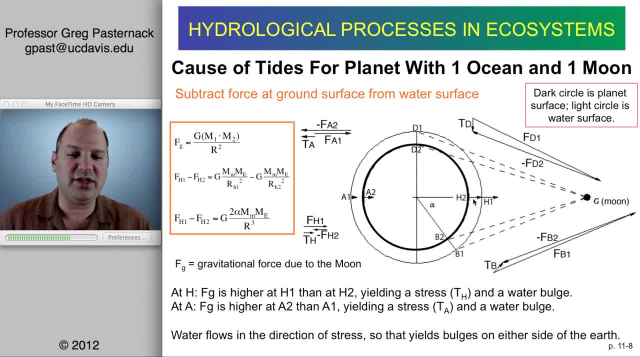 low differential to the area of high differential. and there's two areas of high differential: One and they're both exactly in line with the moon, One on the near side and one on the far side of that water body. Okay, I got through it. 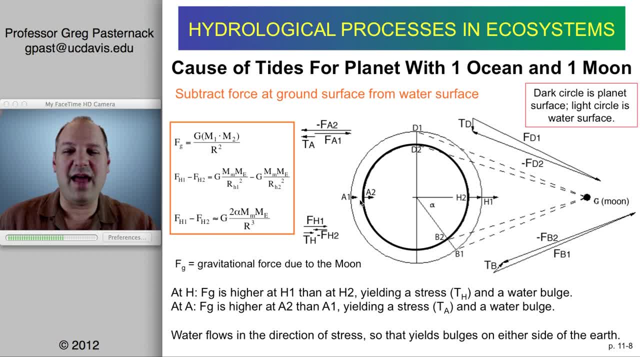 It wasn't as bad as I thought it was going to be, But you'll probably have to rewind that. play it five times, search on the internet ten times and try to convince yourself that any of this makes any sense. So good luck with that. 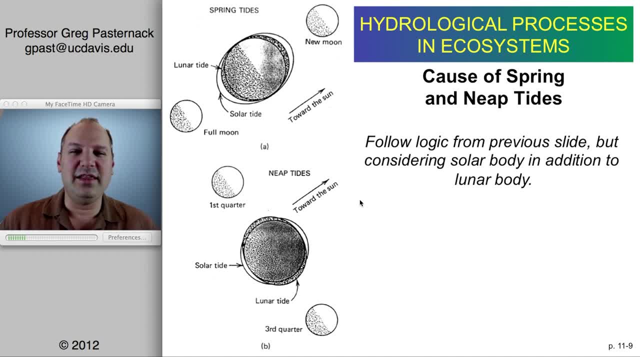 Okay, now let's make it just slightly more complicated. Let's throw the sun into this. If we have the sun, the moon and the earth, now imagine a situation where the sun is direct – let's say – so the sun is like way off on the top, okay, way off on the top. 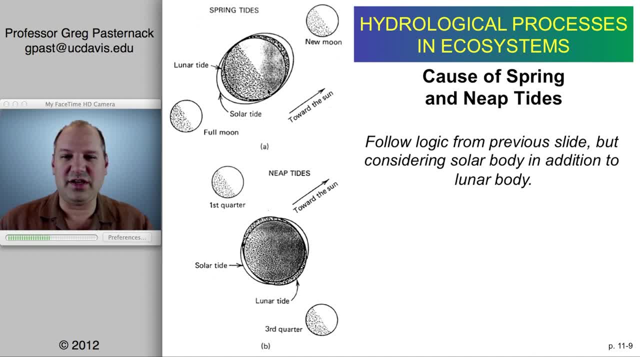 And that's why this is so important. This moon looks sunny on one side, the earth looks sunny on one side and the moon looks sunny on one side. So, whether the moon is a new moon or a full moon, it's all in line with the sun, Everything's. 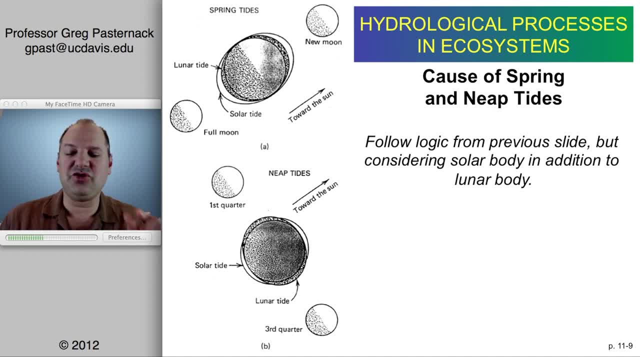 in perfect alignment And, as a result of that, these stress differentials that I was mentioning before are all harmonious. They're helping each other. The differentials are all in line. so you pile up even higher. That means you're going to have higher high tides when the areas of the earth that are 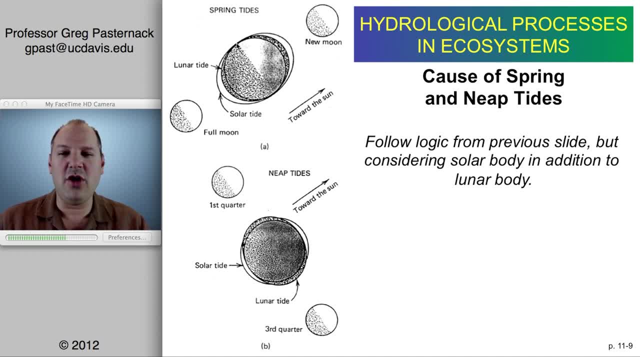 in line with that And lower low tides in the perpendicular position. So, since the planet is moving, it's spinning around, that means that over the course of the tidal cycle, one location on earth is going to experience these different things And I should also – yeah, well, anyway, so you have those tides, That's the daily. 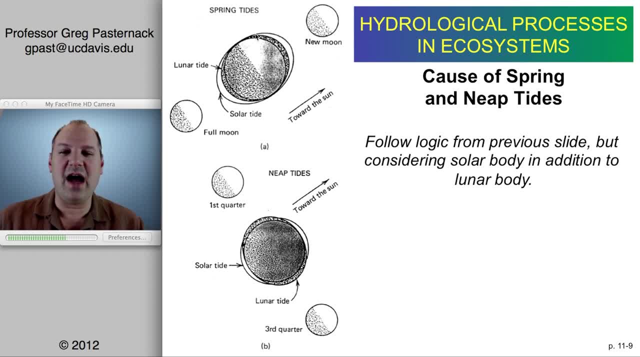 tidal cycle, right. So you're experiencing these strong highs and lows as you go there. So that's the spring tide condition. Now, over time, the moon is going to be orbiting around the sun and it's going to get into the perpendicular position. 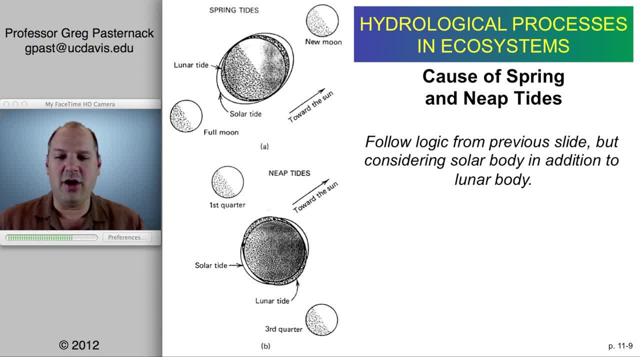 So I see towards the sun, so the sun's over here, and now you have these quarter moons And as a result of that, the bulges are not adding, but you have an independent sun bulge and moon bulge, And so now, as the earth is spinning, the difference between high tide and low tide is not as extreme. 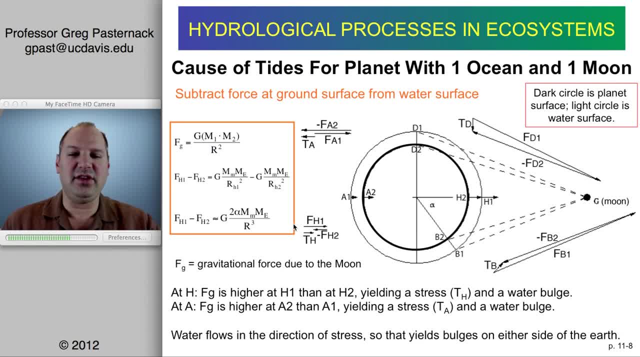 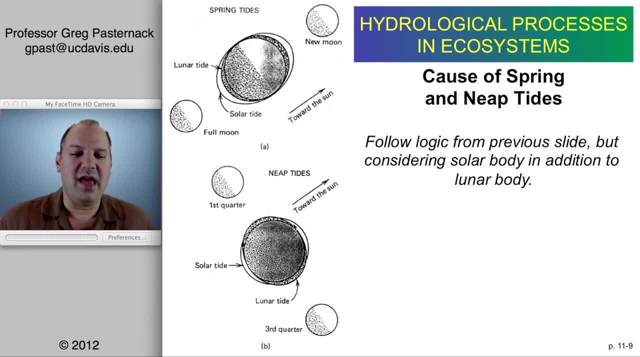 Okay, So we've just taken the explanation of having these force differentials and having water flow from low differential to high differential and applying that with a two-body problem, And what I can tell you is, having now explained this in a video podcast, I'm glad I won't. 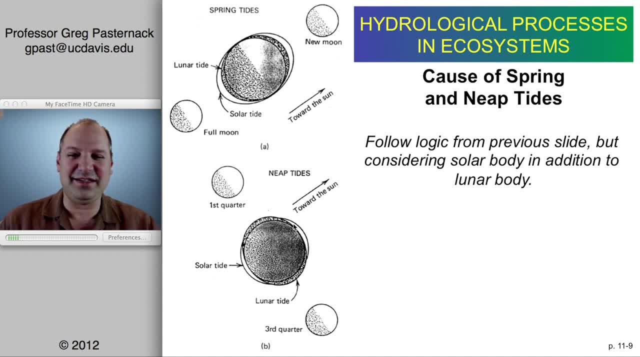 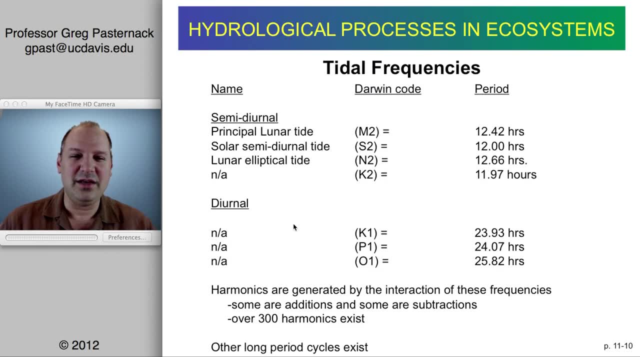 have to go through this ever again in an in-class lecture because it's not fun, But I think it makes sense. It's just force differentials from one location on earth to another. So when you put together all these sources, We have diurnal tides, semi-diurnal tides, the moon and the sun and the earth. 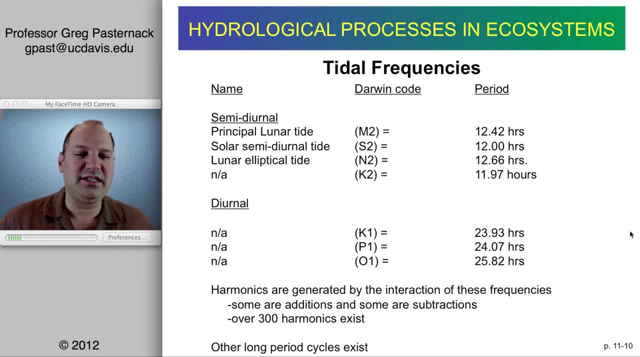 What ends up happening is that we can find different signatures in records of water levels for the ocean, And these are given names M2, S2, N2, and K2.. These are semi-diurnal components that result from periodicities that take place from these. 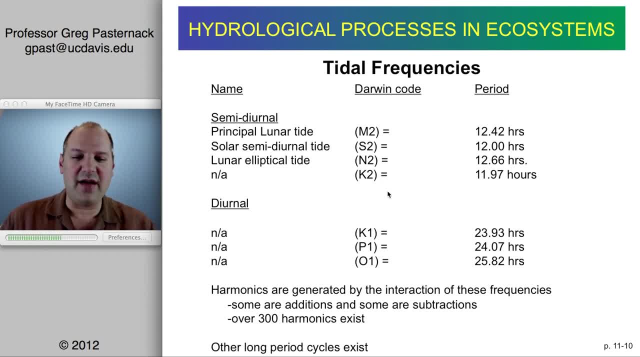 interactions of these celestial bodies. We also have diurnal signals- K1, P1, and O1. And you can see they all have slightly different time frames. that are there. There are also what we call harmonics generated by the interactions of these frequencies. 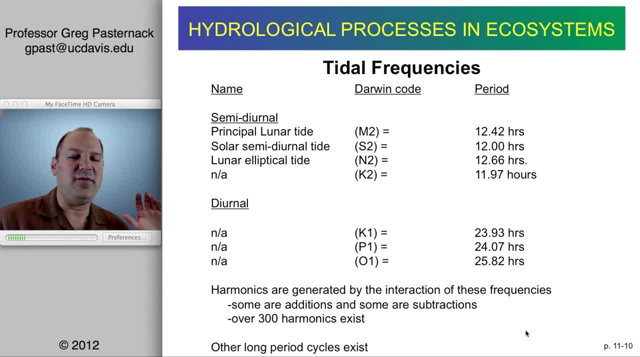 Some are additions and some are subtractions, So it's just like if you were to – let's say you were sitting in your bathtub and you use your hand and you push the water back and forth in the bathtub. If you take your hand and you move it exactly with that, then you can set up very strong. 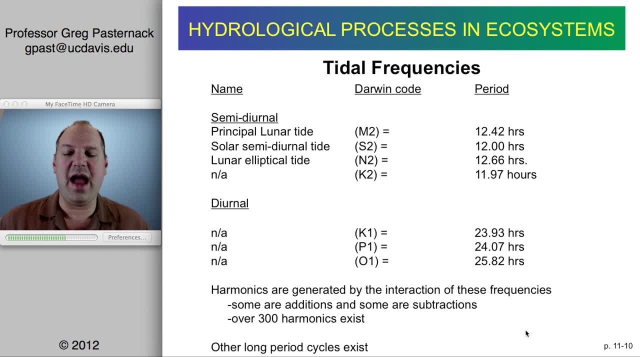 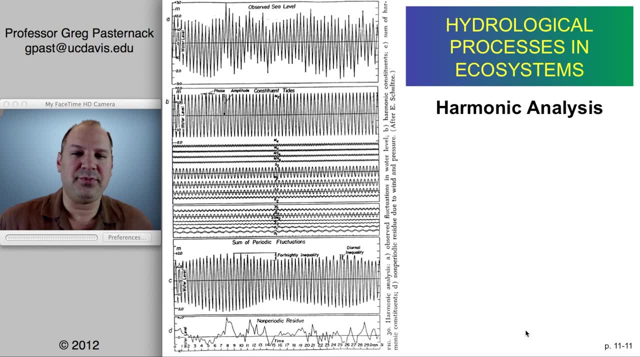 oscillations. However, if you take two hands and you have them go in conflicting directions, you can cancel them out, And that's what this slide is all about, basically. So if we begin with a real sea level record, what you see on the top on the x-axis, is: 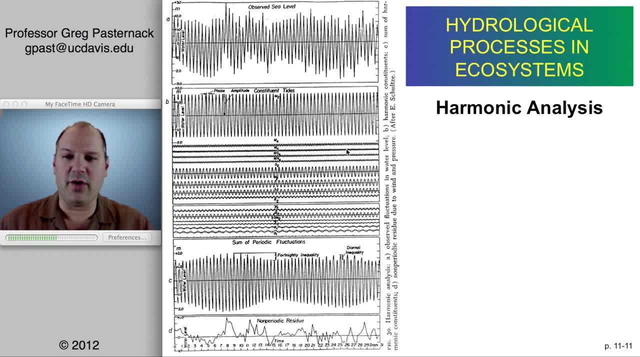 time in days, So it's over a one-month period And you can see water level fluctuates around it. In many cases, when you look at a real record, you don't see – I mean, you certainly see, like the diurnal or semi-diurnal tides very clearly. 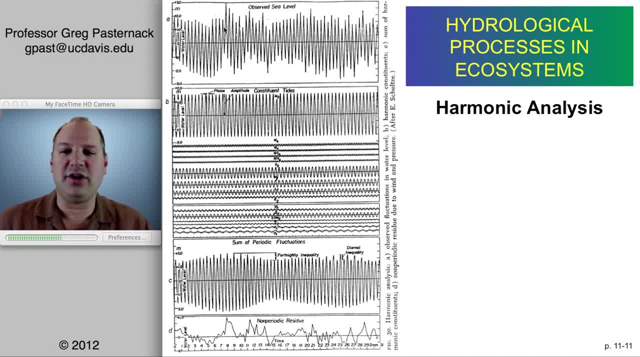 But if you look at a real record, you don't see – I mean, you certainly see, like the diurnal or semi-diurnal tides very clearly, But the other patterns aren't so easy. So there's software that does what's called harmonic analysis. 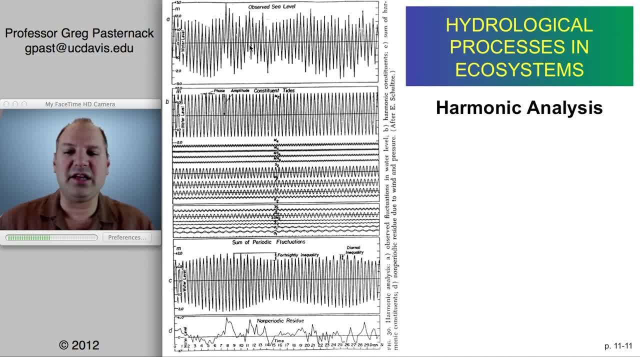 Harmonic analysis is when it takes the raw data and extracts out all these different known tidal constituents, And so you can see here an M tide – well, I mean you can see all these different ones: M2, M4, M6, MS4, S2, and so on. 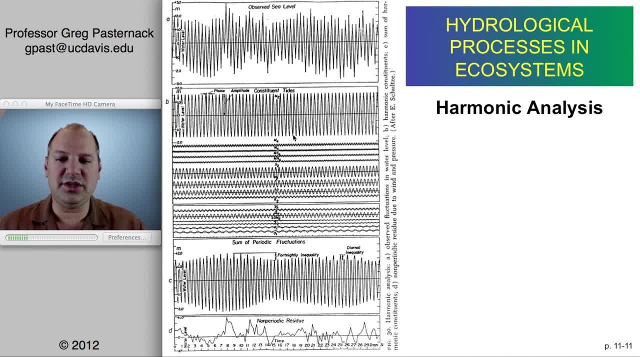 It takes all these out in the appropriate amplitudes, Yeah, And of course the frequencies that those signals have, And then if you look at the sum of all those, you can see that, wow, it still looks fairly periodic. So if you subtract the sum of these harmonic constituents from the observed sea level, 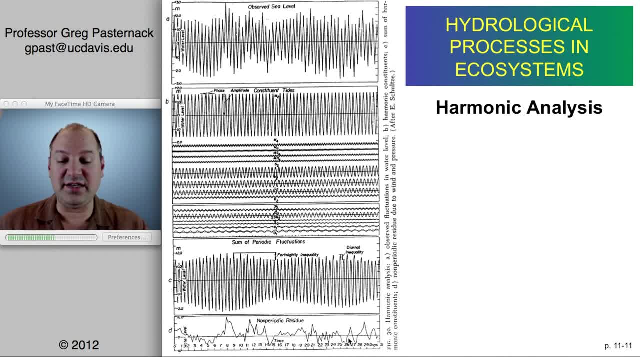 the residual is what we call the non-periodic residue. OK, Let me say this whole slide another way. Observed sea level: something in here is periodic and something in here may be random, or it's just not associated with the tides. 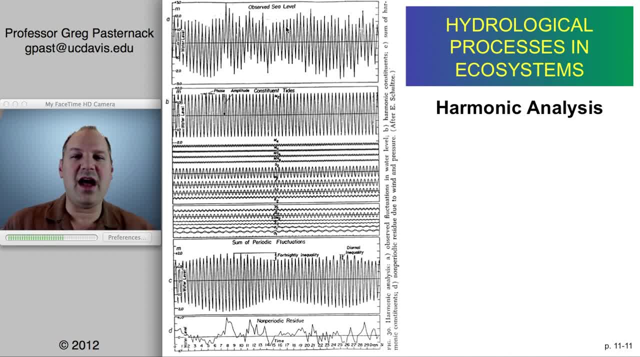 Real data is noisy. Lots of things are going on. Harmonic analysis removes the periodic part of it and lets you get at the non-periodic, non-tidal aspect, which you can then study in more detail And from a wetland hydrology perspective. it's this non-periodic residue that's so. 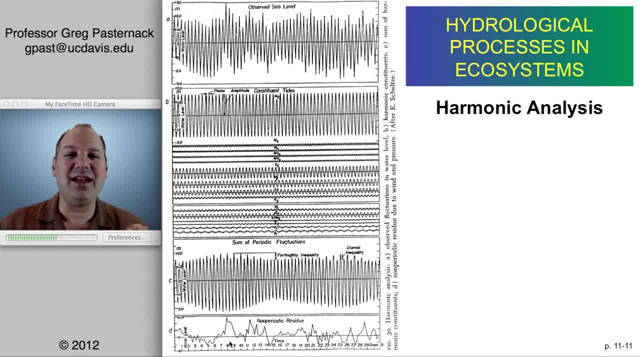 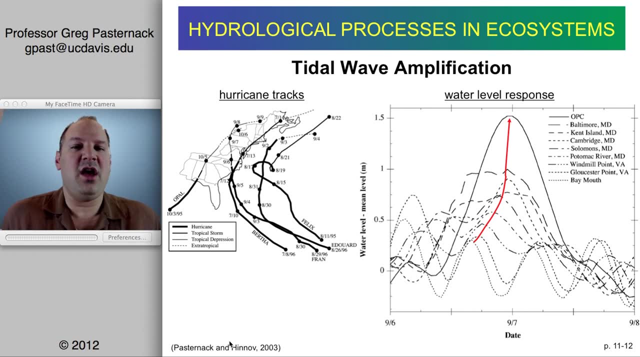 critical because it decides the net non-tidal directionality of flow and storage of water, Yeah Yeah, And storage of contaminants or pollutant sediments or whatever it is. Another thing that can happen is that you can have an amplification of the tidal signal. 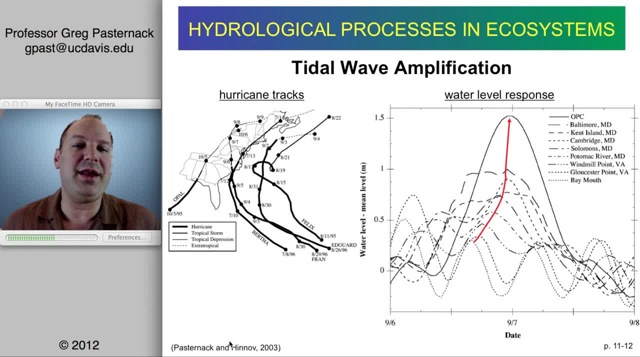 as a result of something like hurricanes or just wind-driven processes. So here's a sketchy map of the eastern United States. There's Florida, And it shows a remarkable one, two, three, four, five different hurricane tracks for hurricanes that took place. 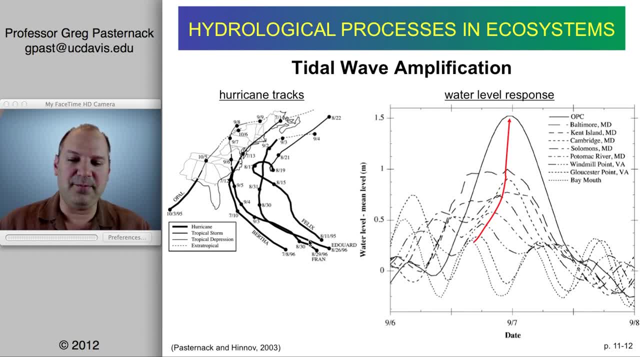 1995, 1996 period. And you can see that these tracks some were more inland, some were more out in the ocean and some went right up the coast. And there was this, particularly this period, on September 6th to September 8th, which would 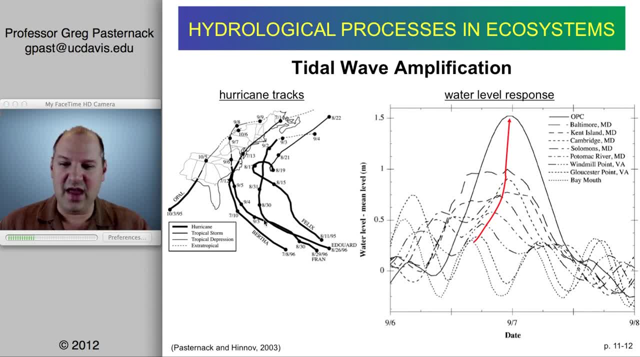 put it potentially here in the track of Edouard coming right up in here, it looks like September 6th, September 8th And you can see that out in the ocean, where the mouth of Chesapeake is, Chesapeake Bay, is this little blip right here by the 713 dot. 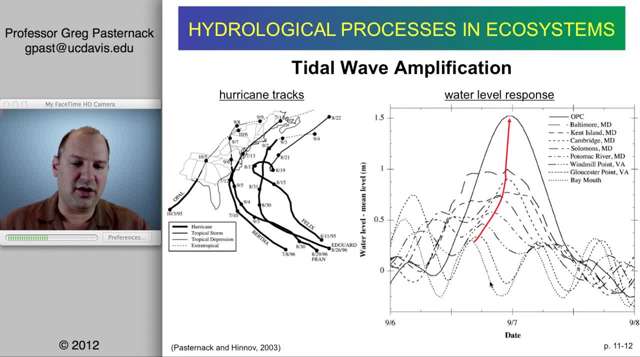 The bay mouth is showing these fluctuations that are here, And then you can see that these fluctuations are growing and growing and growing, until you can see that the largest fluctuation is taking place the farthest inland at this place. that says OPC. Now it's. you can see that OPC was already showing a lot of these are showing changes. 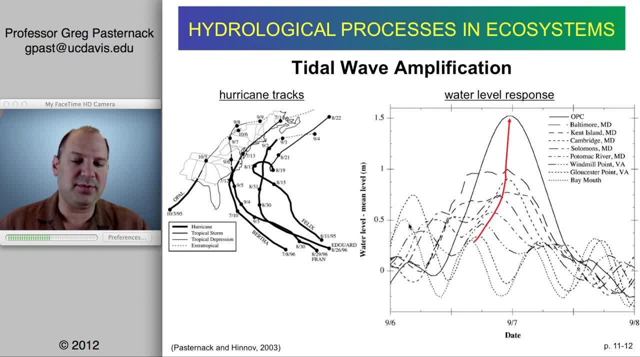 before we see this main event. So there's probably a combination from the previous high tide coming in and this current one. You can see, though, that there's a cumulative effect, or what we call an amplification, as you go inland, And I should say that's because you're taking a lot of water, you know a lot of water with. 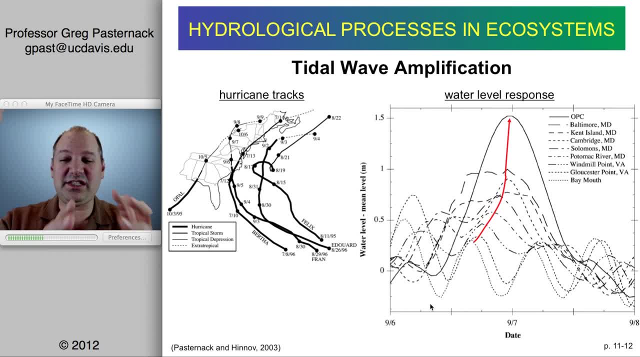 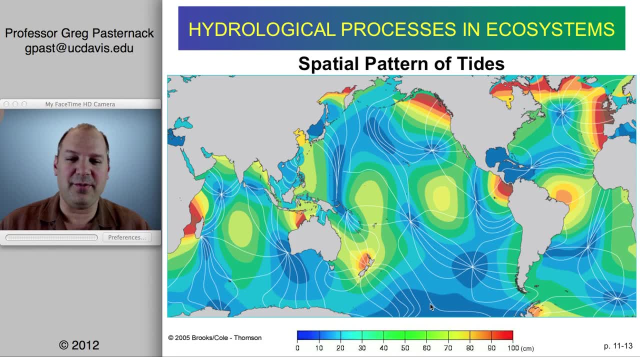 this very small elevation change and you're shoving that into a very small hole and as it goes in, then that's raising the water surface. So that's what that's happening there. Here's a map of the whole world. The continents are shown in gray and the ocean is shown in these bright colors. 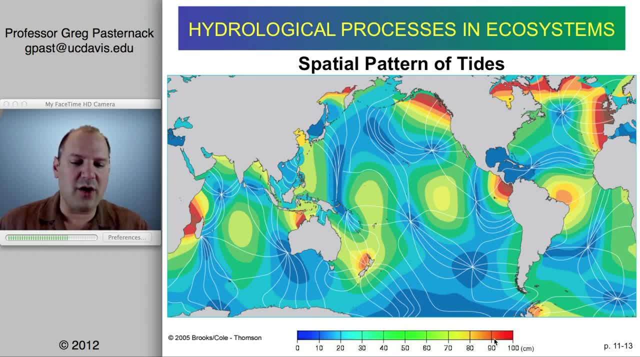 Relative to mean sea level. red indicates higher water levels and blue indicates lower water levels. And what this map is showing is the complex spatial patterns where you have net higher water levels or lower water levels, because water is doing this amplification process. You know, we don't just have a water world. 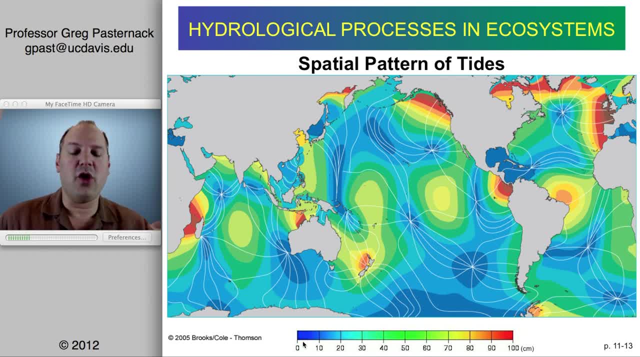 We have continents And tides have to ebb and flow around these land masses and that forces this complex pattern that you see. The white lines here show the time differential of one hour between high tide at one location and another. So everything along this line is seeing high tide at the same time, but from one line to 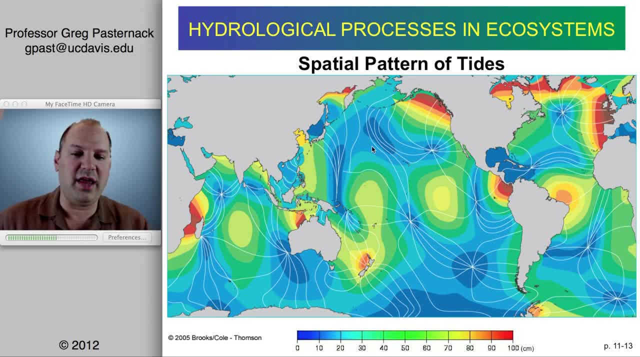 the next. you're seeing high tide at an hour earlier or later, So you know from here Whatever the tide is, Because you know the tide has to tidal wave has to propagate across the ocean, and so that takes time and it's so many hours later. 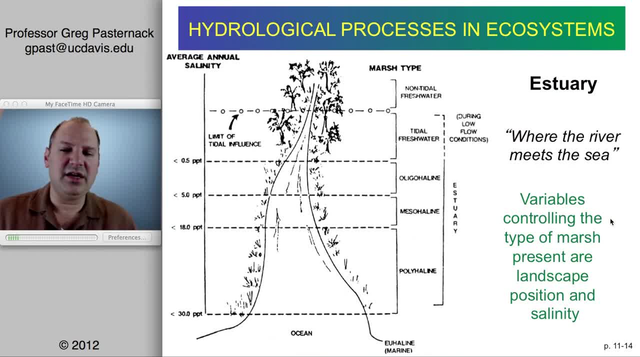 Okay, That's the explanation of tides. Now let's move into the coastal context. So remember, from the hydrogeomorphic method, we often look at the geomorphic context, the hydrology and the hydrodynamics. I had to present the tides because, of course, from a hydrological standpoint, as we'll get. 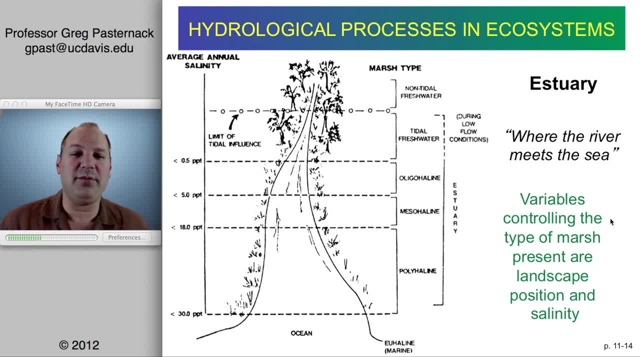 into later. The tidal exchange is the dynamic, The tidal exchange is the dynamic, The tidal exchange is the dynamic And the geomorphic process is usually the predominant component by far. So that was an important part. Now we're going to turn back and look at the geomorphic context of the system. 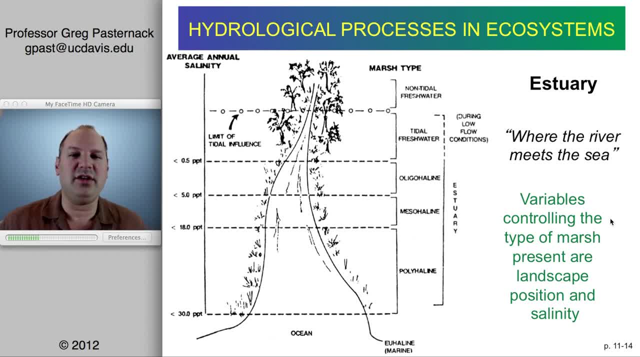 And I'm going to be focusing on estuarian wetlands relative to coastal marshes. A lot of the things that we have in coastal marshes are also represented in this lecture, but there's a lot more diversity of processes in an estuarine setting, and so I'm going to 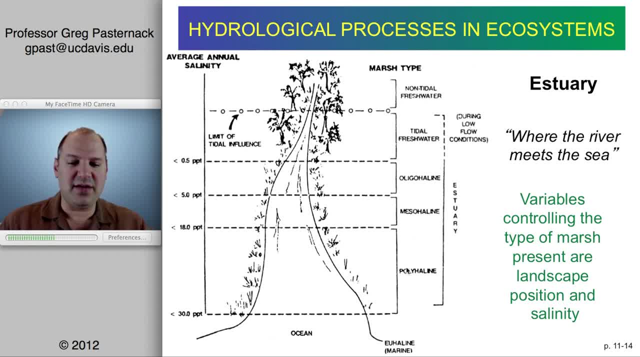 focus on that. So here's just a generic schematic of an estuary, nothing more than where the river meets the sea. Generally, you have, as you've already seen, tidal amplification as you go up in there, but eventually you reach a point where there's no more tidal signature, although that can be quite far. 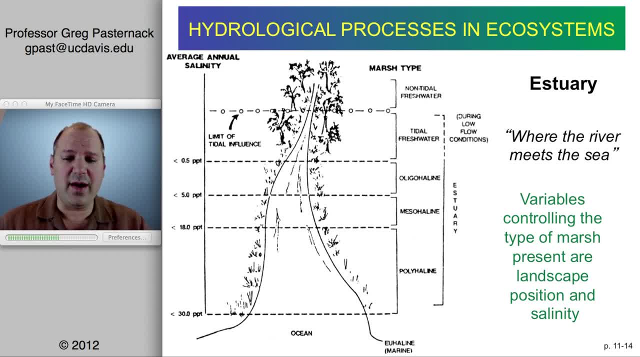 inland. In addition to tides, you also have a gradient in salinity going from about 30 parts per thousand at the ocean to less than half a part per thousand in the freshwater. tidal influence, and then eventually, you get to an area where not 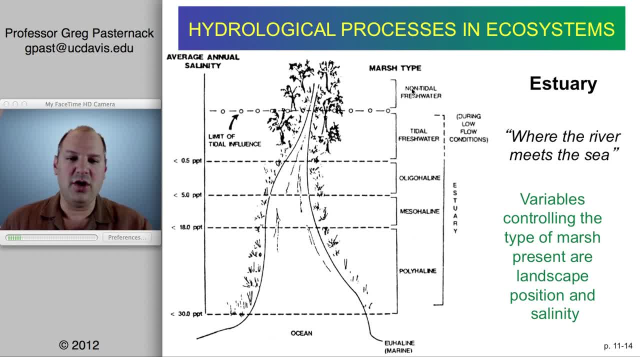 only is it not salty, but there's no more tides. So you have non-tidal freshwater zone, which we'll be looking at in the next chapter. tidal freshwater, oligohaline, mesohaline and polyhaline just mean getting stronger and stronger in terms. 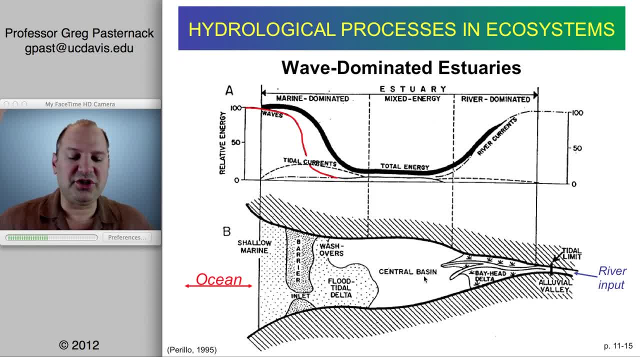 of salt conditions. So there's three broad-based processes that affect coasts, and especially in an estuarine context. These are waves, tidal currents and river flows- or river currents Depending on the combination of those three- interacting with the landscape. 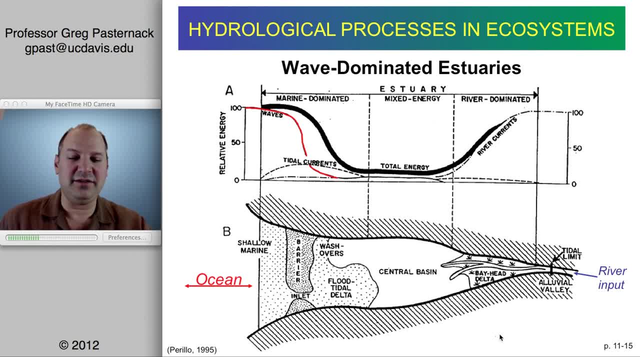 morphology of the estuarine basin. you get a characteristic signature to the system, both in terms of energy processes and features. So, as you continue to explore the system, some of the things you can do as you progress with your work. you can go to the beach. You get a characteristic signature to the system, both in terms of energy processes and features. 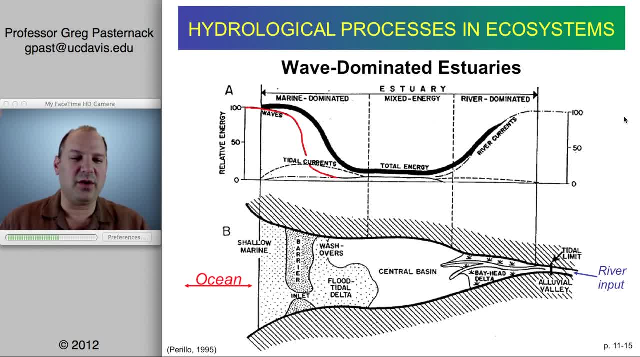 and features. How does this work? Well, in these diagrams, the far right is where the river is flowing in, So the river is flowing from right to left, and then you have the ocean on the far left and you have that bidirectional exchange, from left moving to the right. 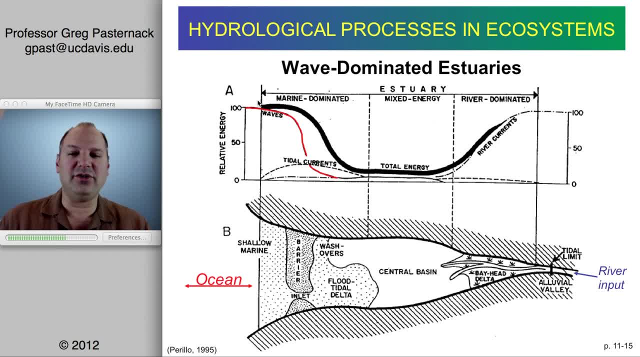 So this is an example where you have high wave energy in the ocean, which is characteristic here in California: High wave energy. what do waves do along a coast? Well, they cause what we call longshore transport of sand, moving sand generally in one direction, up and down the coast. 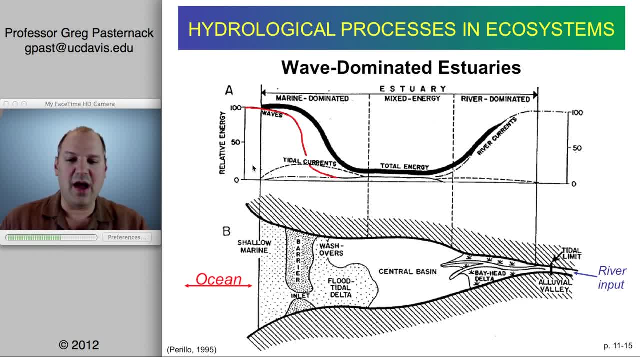 although there can be more complex patterns. So, as that sand, when it reaches the mouth of an estuary, if wind-driven waves are strong enough, then they'll just carry those sands across and they'll just block it off. And this is a photo that's showing a complete blockage where you have a barrier. 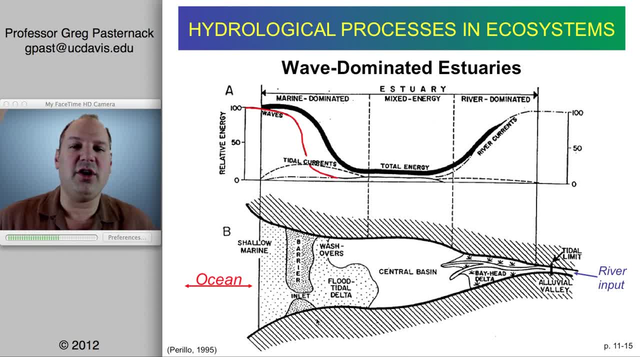 and then a very small barrier. These are ubiquitous here in coastal California, Whether it's the mouth of the Russian River or Guadalajara, the Faro, you go up the coast or down the coast, you can see these barrier inlet systems all the time. 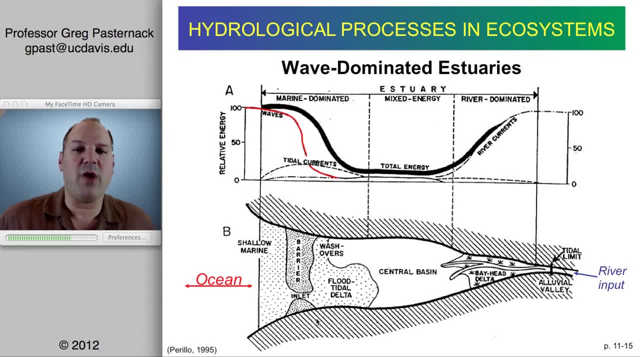 So throughout the year, you can have rougher sea conditions. What matters, then, is: what's the river input at the other end? In a semi-arid to arid climate, river inputs may be quite small, and so you have a lot of energy right at the transition from the alluvial valley to the estuary. 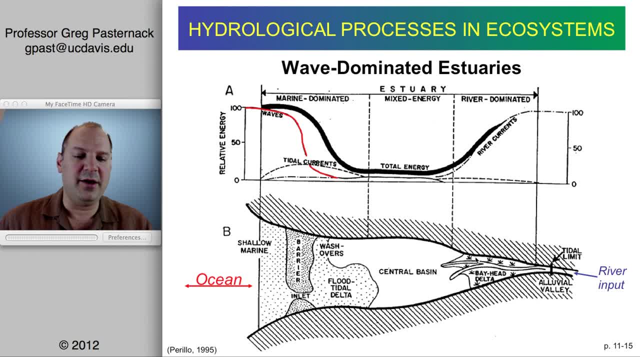 but most of the energy will be lost right there and you'll get a deposition of sediment, potentially forming a delta, like you see. there There could be a large central basin or a lagoon that is relatively quiet In modern times. that may be a hypoxic or anoxic setting in which you have a lot of pollution. 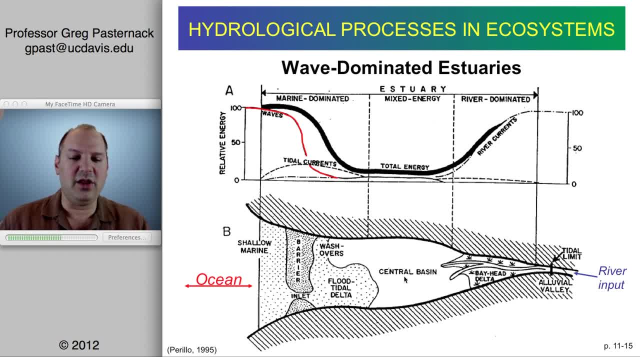 or fish health problems, But it's generally a low energy climate. So in this context, we have a wave dominated system, where the coast is dominated by waves and the river has a relatively minimal influence. Now what happens if the river is not small? 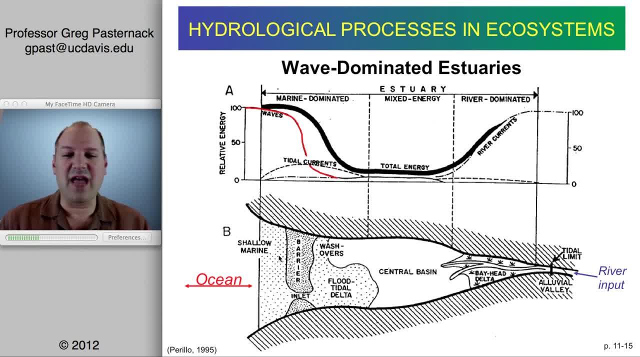 Like, let's say, you have relatively little waves, little tides still, and the river is just blasting through. Well, if that's the case, you probably don't have an estuary at all. The river is completely filled in and it's pushing sediment out of the estuary. 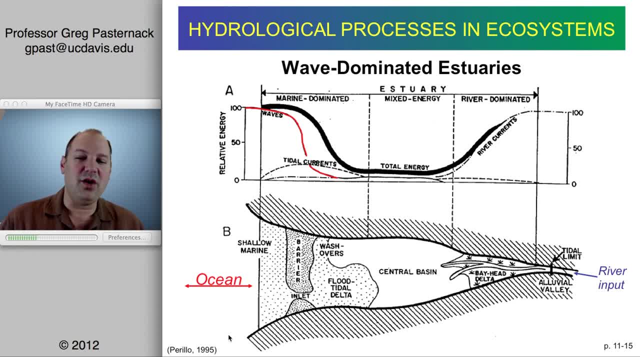 So you get sediment out and you get what's called a delta. A delta, you know, whether you think of a delta as estuary or not is a little bit iffy. I mean, there are certainly tidal gradients and salinity gradients throughout a delta. 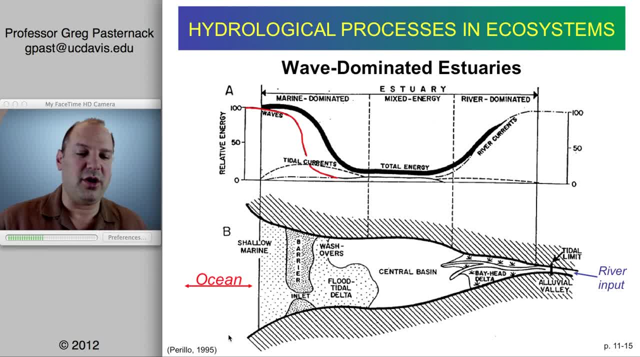 but a delta is a whole other kind of landform compared to estuaries. So an example of that would be the Mississippi River Delta, the Nile Delta. You know, those would be two classic examples, but there's plenty more. And so that's if the river is pushing straight out. 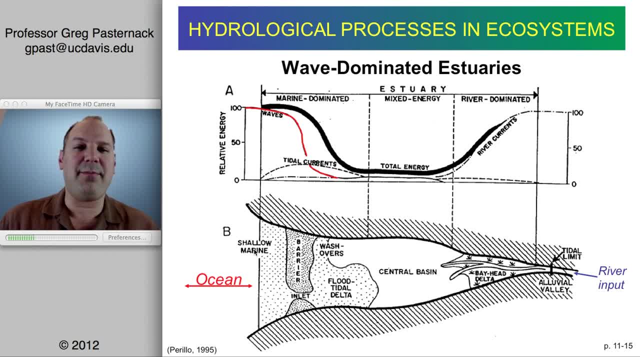 So I'm not going to show that end member, but I'm going to show you a little bit of an example of a river dominated estuary. So river dominated would not be an estuary, it would most likely just be a delta. But you do have small deltas in these wave-dominated estuaries. 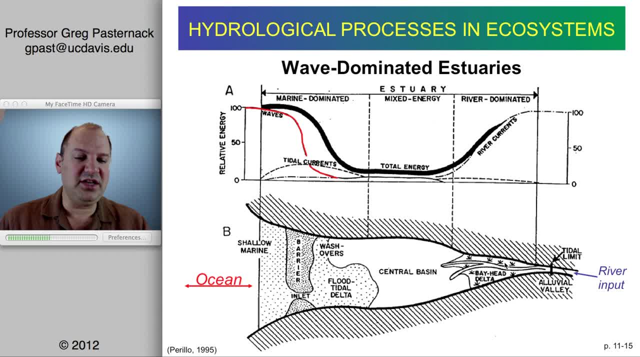 And you can see from a wetland context- and this is, after all, a video podcast about wetlands- you can see the wetland is occurring on that relatively small Bay, Hat Delta. It's unlikely to have much on the barrier, but you could have some salt marsh in the flood tidal area. 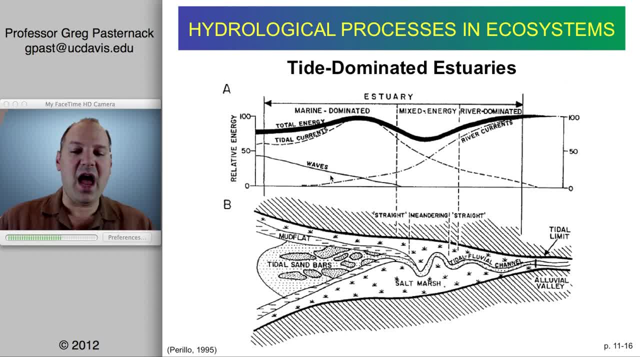 This is a case where you have a dominance of the tide. So now you can see that the tidal energy is relatively high, more than 50% of the energy. There's still high wave energy at the mouth, but it diminishes as you go inland. 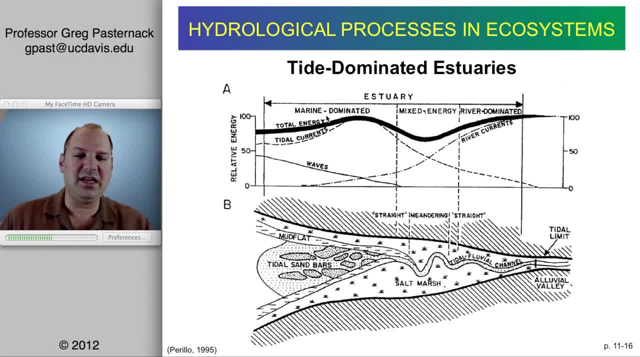 And there can be quite high river currents, But the thing is the tidal currents. And so, since tides go in and out, whereas the wave tendency was to block the river mouth with sediment, the tides are now going to push in and out and create these longitudinal sandbars. 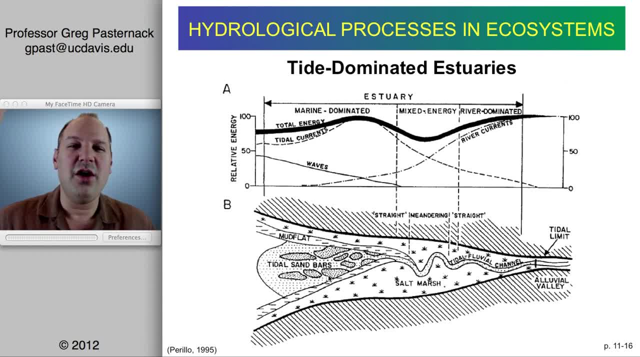 Now these are the sandbars that, in the colonial era, were responsible for causing shipwrecks. So, whether they're merchants or pirates, or naval vessels of one kind or another, trying to navigate into tide-dominated estuaries was the bane of the existence of these mariners. 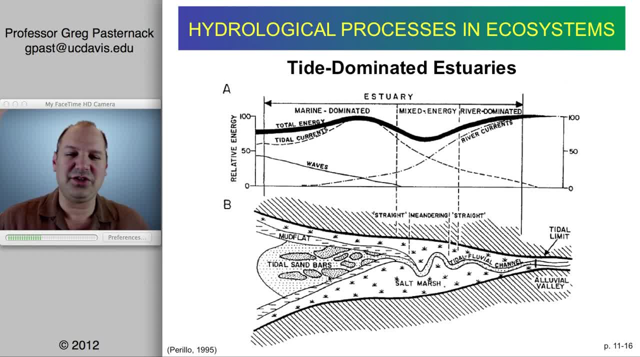 And a classic example is the Delaware River Estuary. The Delaware River Estuary is well known to be a source of a lot of lost golden coins, And so there's a lot of coins that can wash up, and there have been a lot of shipwreck stories on the Delaware River tide-dominated estuaries. 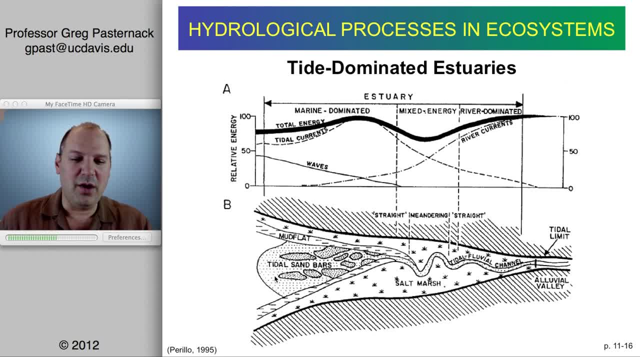 So if you're into that sort of thing, check that out. When you look here, what you can see is that the sandbars themselves- because they're shifting around, they can't allow vegetation to establish, But you can see that tide-dominated estuaries develop vast complexes. 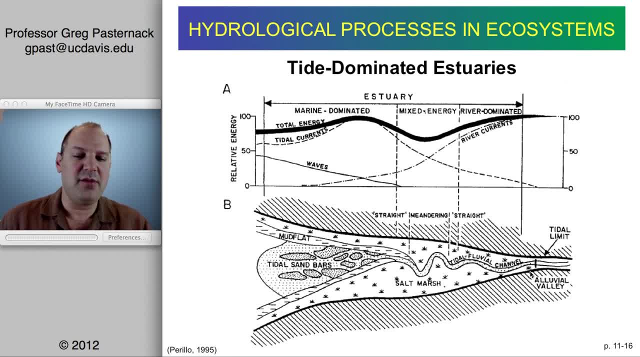 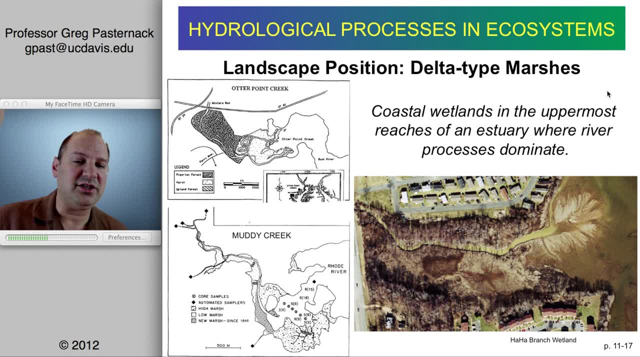 of salt marshes throughout the entire system. So if you look here, you can see that there's a lot of sandbars that are moving across the central basin peripheral to the channel. Now, regardless of where you are in an estuary, let's move from the estuary context. 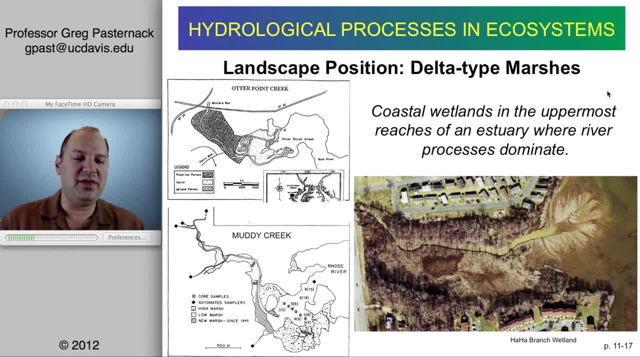 to the scale of an individual wetland. At the scale of a wetland generally, there are two kinds of wetlands that you commonly see reflecting landscape position. One are the delta-type marshes. So if we go back, you know, here we have this wave-dominated estuary. 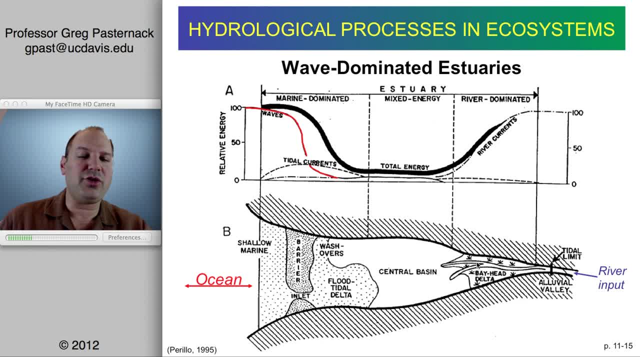 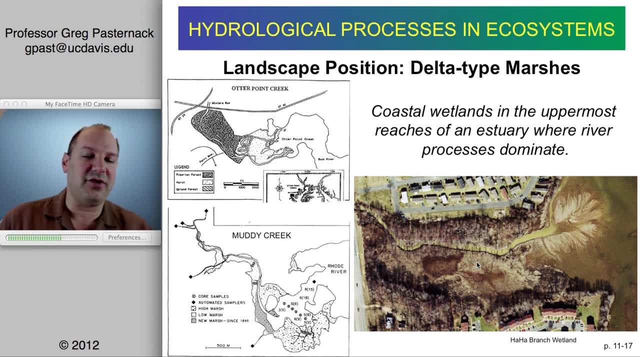 Wave-dominated or not. if you're in an area where the river is pretty far away from the ocean because it's a very long estuary, and if there are substantial sources of either natural or anthropogenically influenced sediment contributions, then you can see you get a delta. 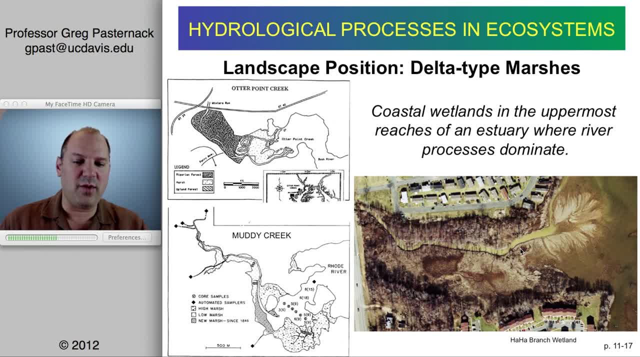 And so you see, this river is coming in from left to right. There's a wetland complex that's completely filled in this sub-estuarian area, And then there's a, you know, like an exposed, sandy, muddy flat that's out here.